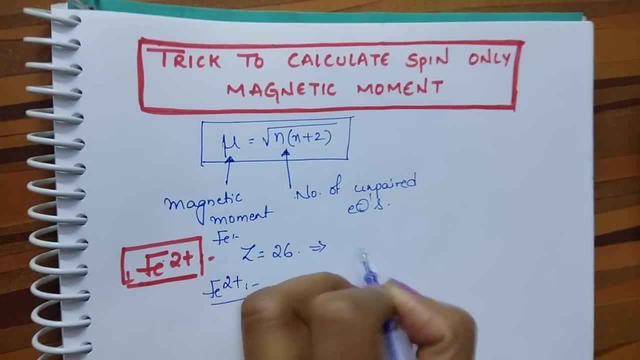 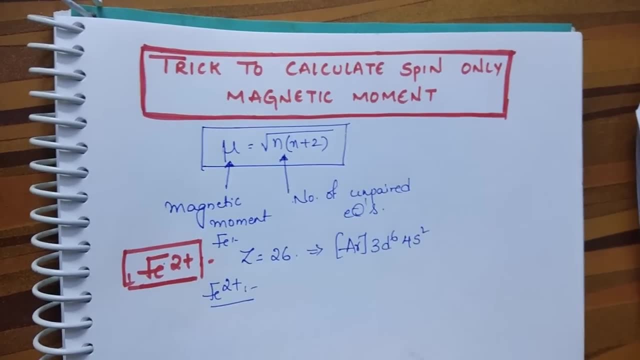 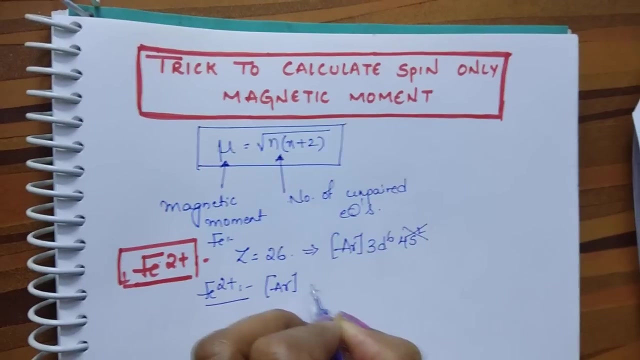 in plus 2 state. First, what you do is write the electronic configuration of Fe argon 3d6 4s2.. It is in plus 2 state, So remove these two electrons, Then its electronic configuration is argon 3d6 4s2.. 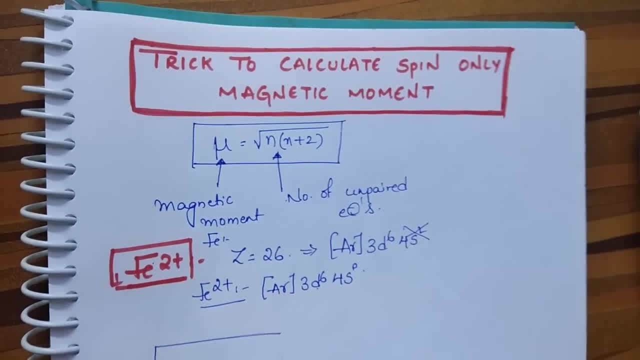 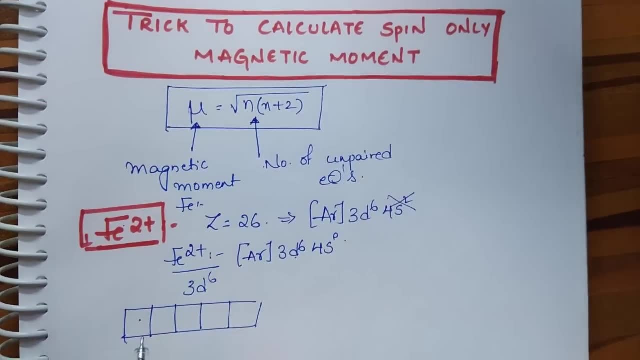 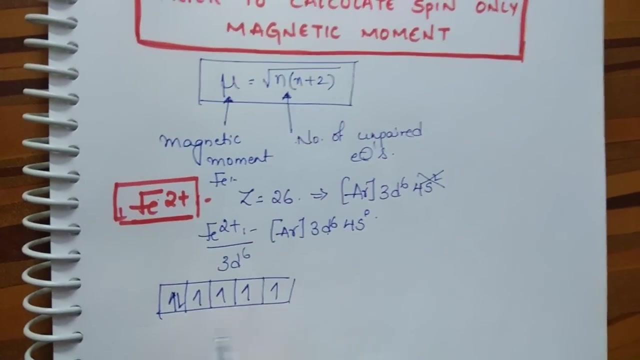 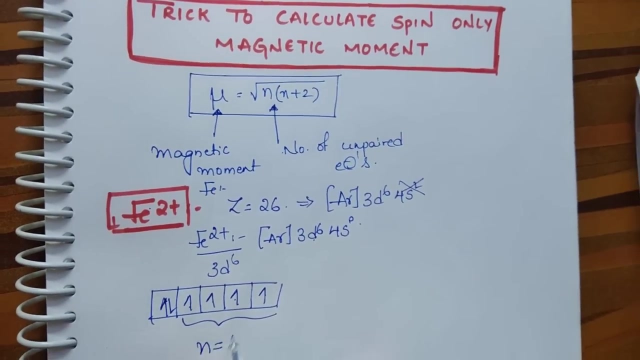 Now take this d6 orbital. How many electrons are there? 6 electrons are there. Write this: 6 electrons. Now, how many unpaired electrons are here? Single electrons are there: 1, 2, 3, 4.. So n value is 4.. If n value is 4, then magnetic moment mu is equal to 0. Now take 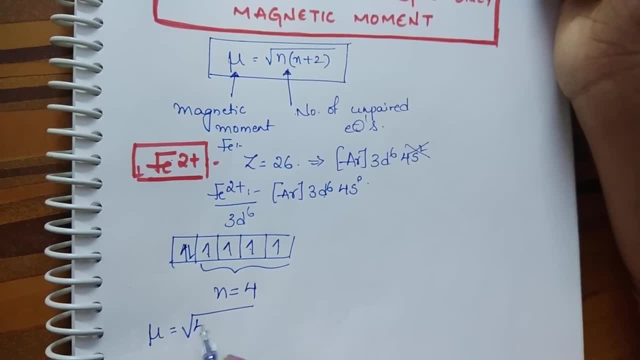 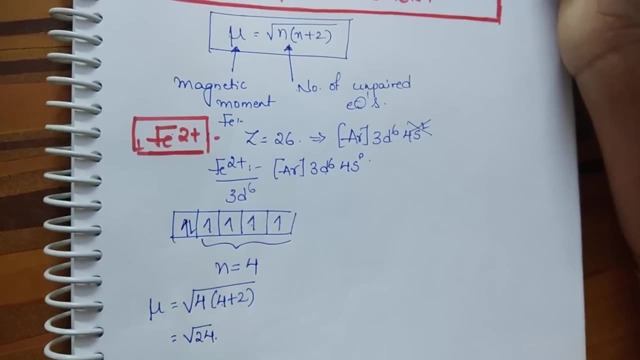 these two particles. It is equal to square root of n into n plus 2.. So 4 into 4 plus 2.. 6 4s are 24. Here you see square root of 24.. So its square root of 24 bore magnetons. 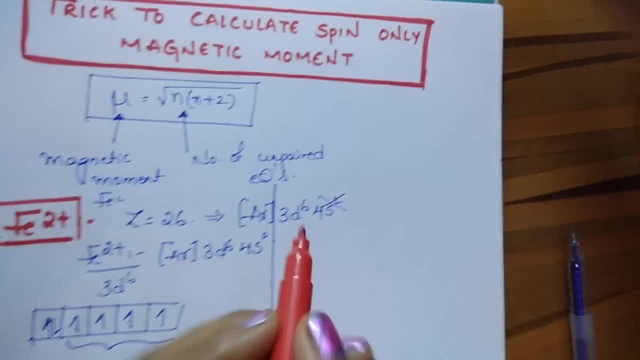 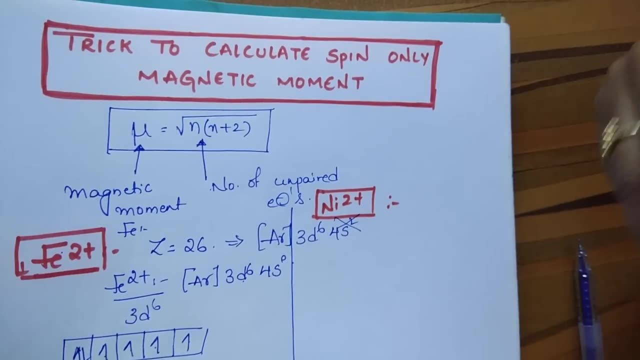 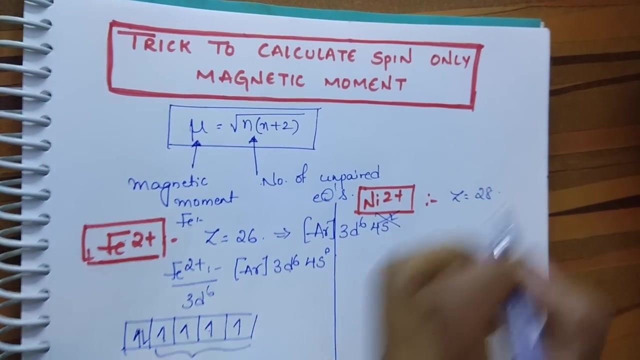 Now find for Ni2+. Find the magnetic moment to Ni2+. Just enter the magnetic moment. This is the magnetic moment which we wrote there. Let us write it here. Po didn't go well. just what is atomic number of nickel students? atomic number is 28 and its electronic configuration. 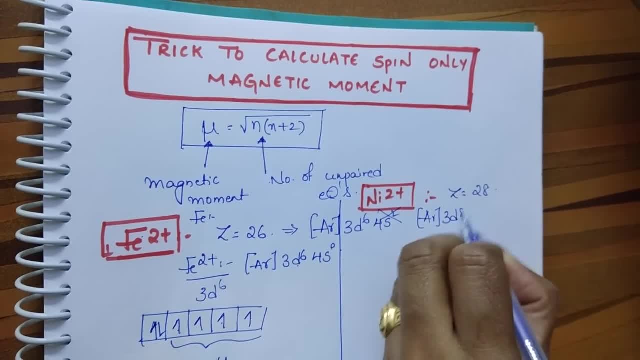 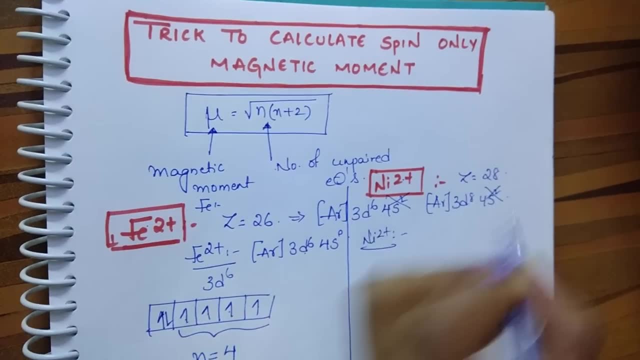 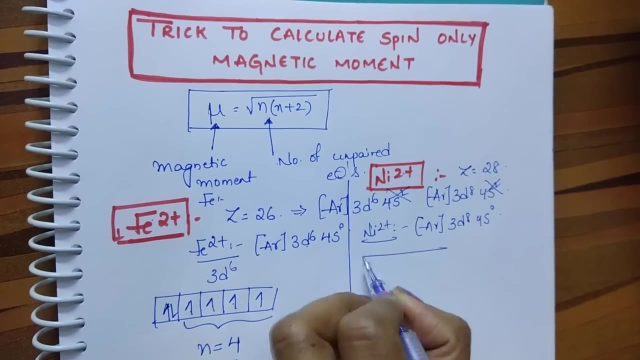 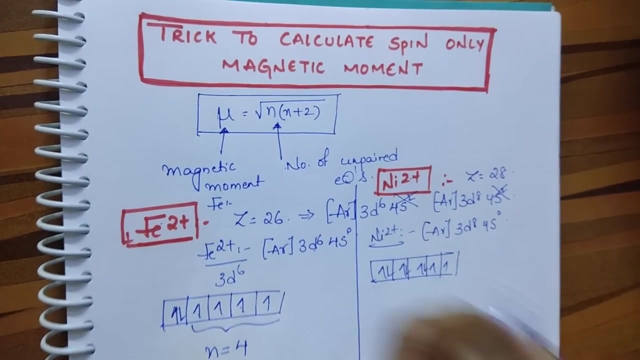 is argon 3d8 4s2. here nickel is in plus 2 state, so what you do is remove the two electrons. then you get argon 3d8 4s0. just take this d orbital and fill the electrons. 1, 2, 3, 4, 5, 6, 7, 8 are there. 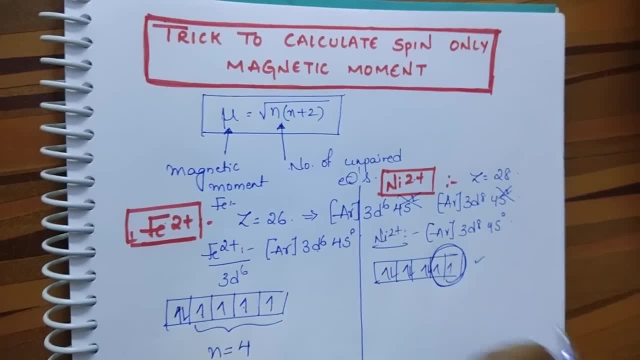 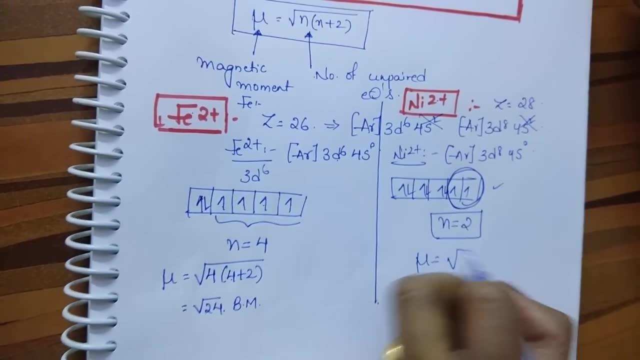 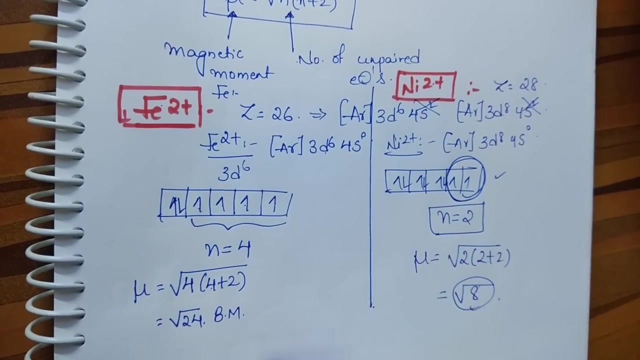 now how many unpaid electrons are here? number of unpaid electrons are 2. if number of unpaid electrons are 2, then mu is equal to what? 2 into 2 plus 2, then it will be how much four twos are 8, square root of 8. now time for the trick: square root of 24 and square root of 8. taking the: